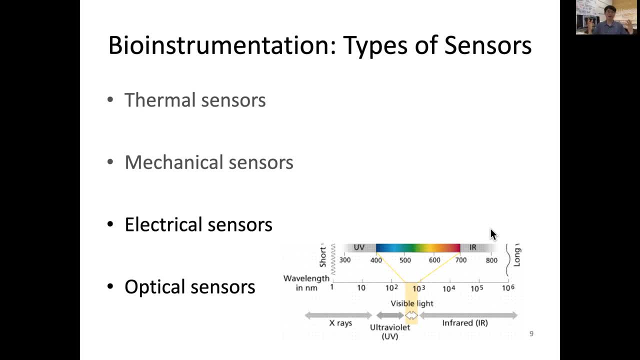 All electromagnetic waves are produced by electron acceleration, especially periodic motion. So you can see from UV, ultraviolet, to visible light, which is about 400 to 700 nanometer wavelength range, and IR- it's infrared range. So our visible light is only a very narrow part of the spectrum. 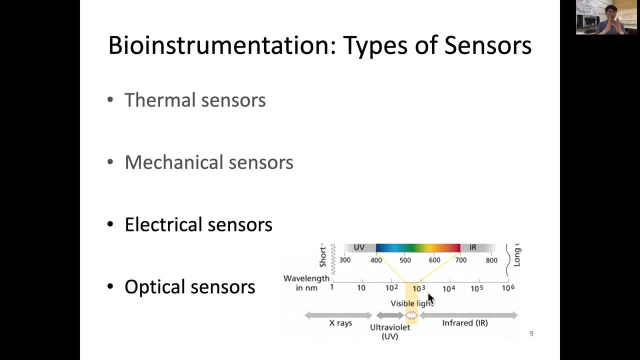 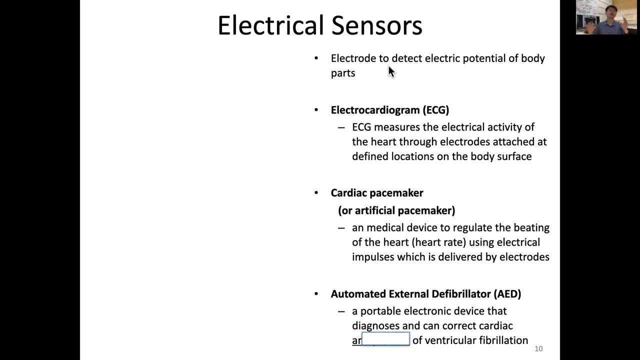 which can be visualized and recognized by our eye, especially the retinal system of cones. So let's start with the electrical sensors, So we can use electrode to detect electrical potential of our body parts, especially like heart, That we call as electrocardiogram or ECG or EKG. 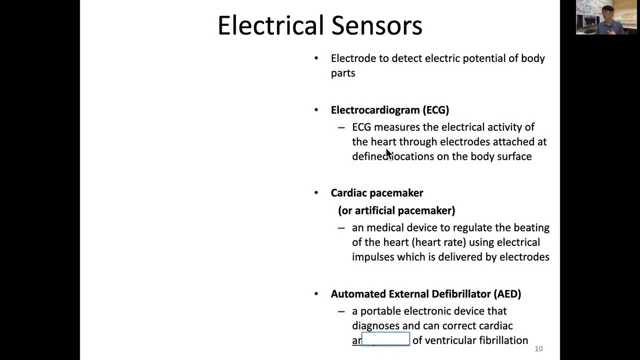 That ECG measures the electrical activity of the heart through electrodes noninvasively put on the surface of defined location of our body. So, such as you've already seen, this ECG And the next is the cardiac pacemaker, or we call artificial pacemaker, because our heart has its own pacemaker called SA node and AV node. 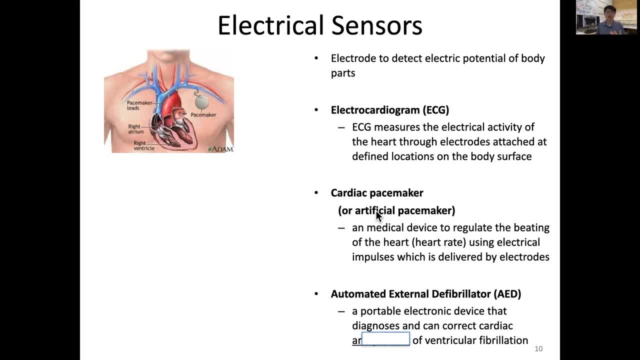 We have developed this artificial pacemaker, which is a medical device to regulate the beating of the heart or heart rate, using electrical impulses, which is delivered by electrode. You can see here a pacemaker is implantable and that electrode is going through these veins and to right atrium and right ventricle so that it can provide a regular heartbeat for those who has a patient. 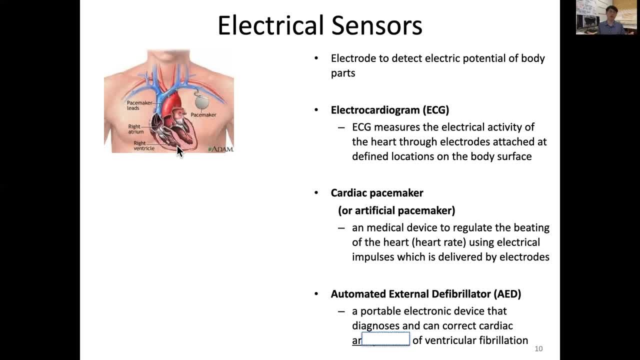 Those who has a problem with the heartbeat, or we call it as a arrhythmia. So the next is about defibrillator. So when a person has a cardiac arrest, so that is an emergency case and we can use external electrical shock to reset the heart and regain the proper rhythm.